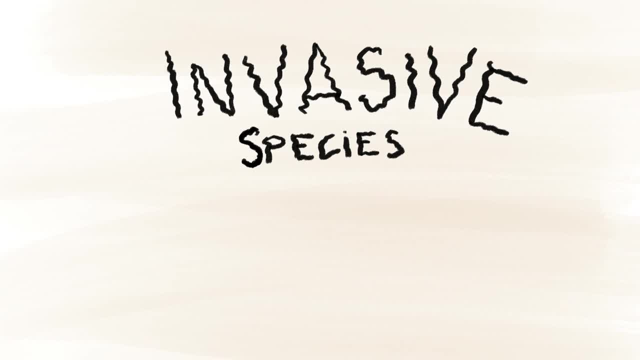 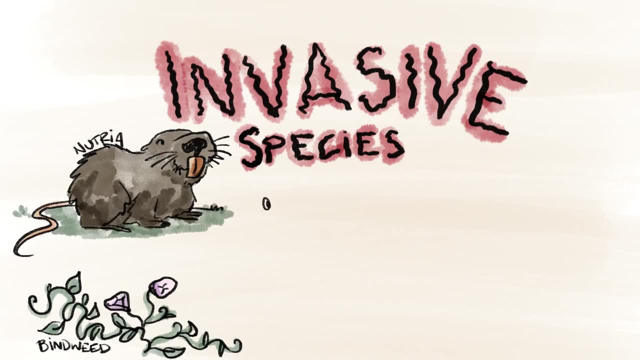 Invasive species. You've probably heard the term, but what exactly does it mean And how is it different than terms like non-native species or pests? Great question. Come along with us as we explore these different terms. First, a little sneak peek into invasive species. Invasive species include plants and 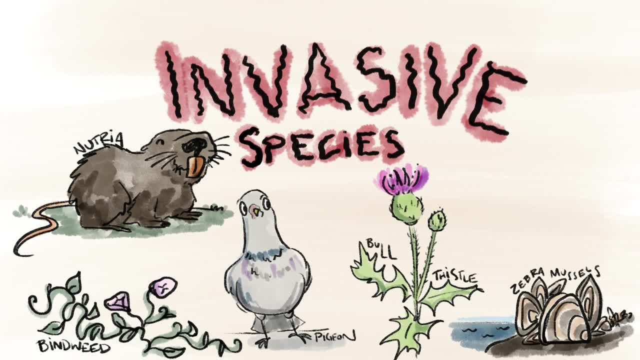 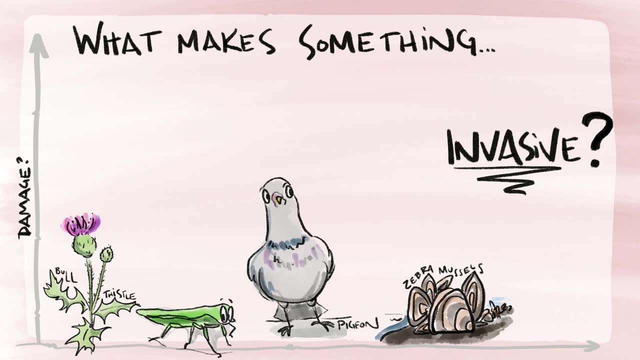 animals both in water and on land. They are found in many places, including national parks. They threaten the Park Service mission to preserve unimpaired America's natural and cultural resources. So what makes a plant or animal invasive? Does it have to do with a certain amount of damage, or is it just a species that? 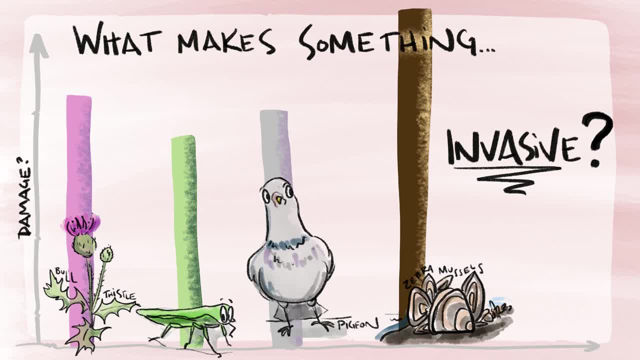 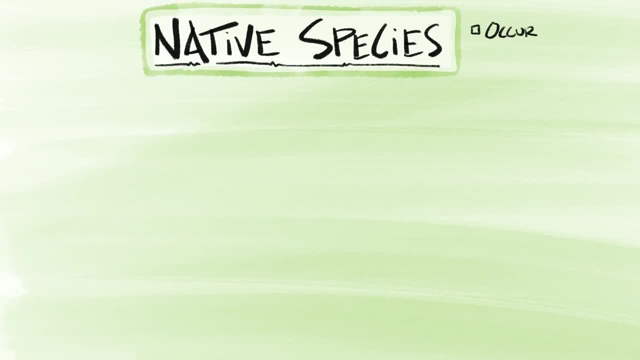 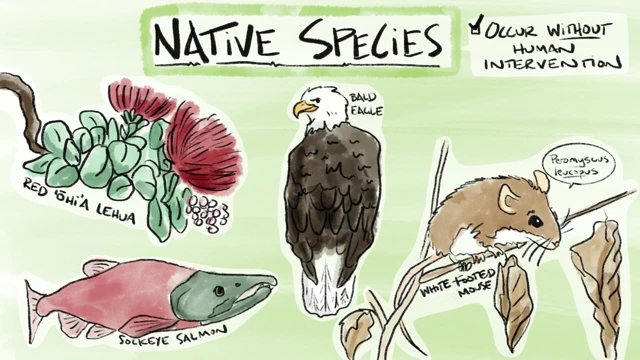 left its own habitat. Let's talk about some other definitions, like native and non-native, before we dive into the big question. Native species: These are all organisms that have occurred, now occur or may occur without human intervention. One example is the white-footed mouse. It's native throughout the eastern United States. 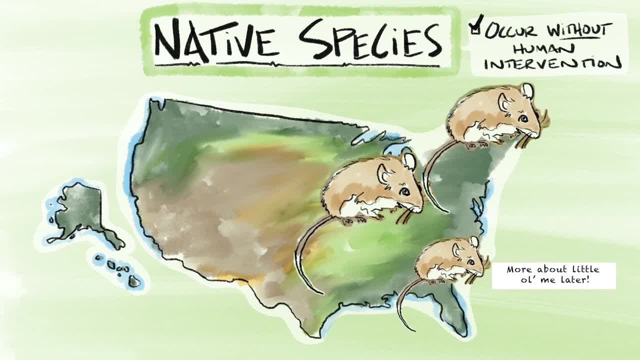 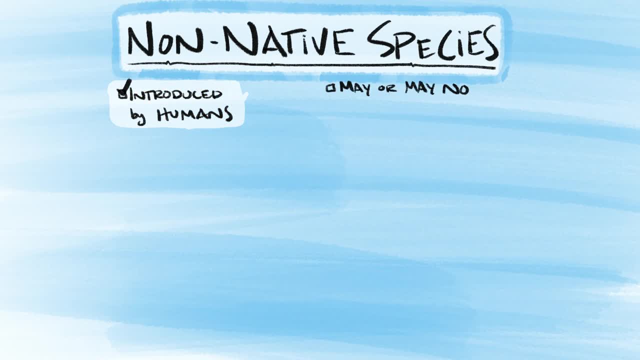 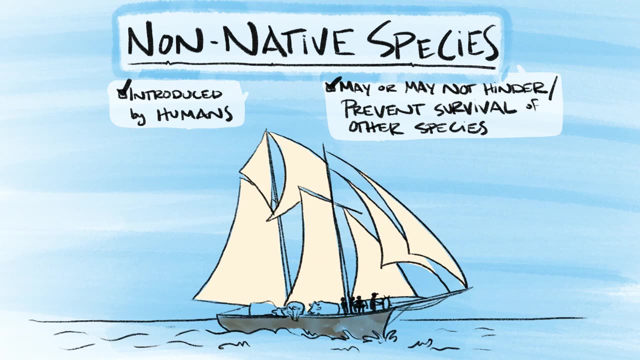 When found in nature, the mouse is an integral part of the ecosystem. Non-native species: These are species that do not occur naturally in an area, but are introduced as a result of a deliberate or accidental human activity. Most importantly, they exist where they have not naturally occurred and may even be. 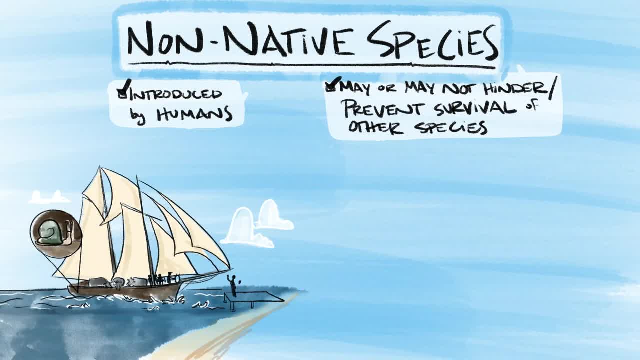 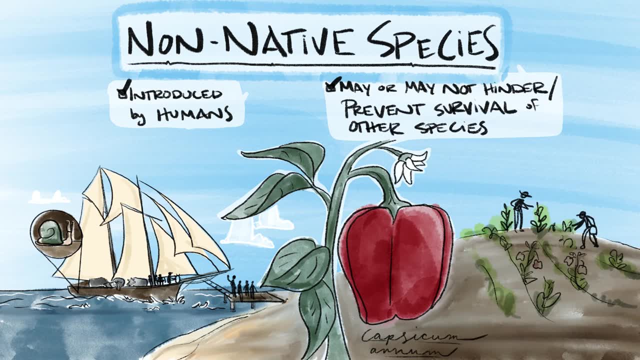 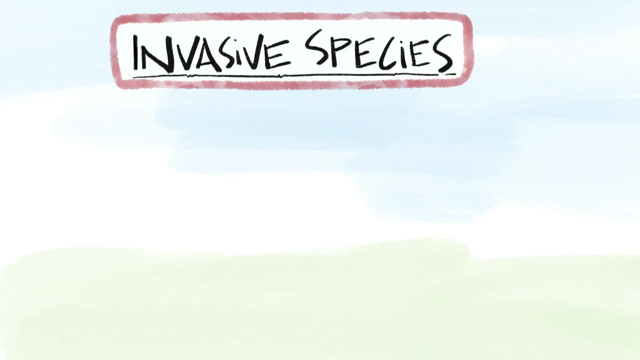 considered beneficial under certain circumstances. One example you may recognize is the bell pepper. It's not native to the United States, but it currently presents no threat to native plants. Now it's finally time to explore invasive species. Invasive species are non-native species that cause harm to the environment. cultural. 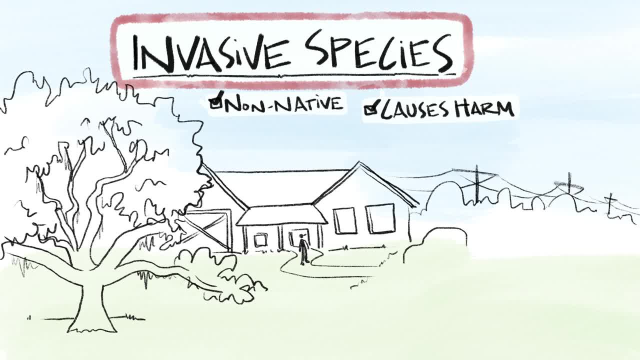 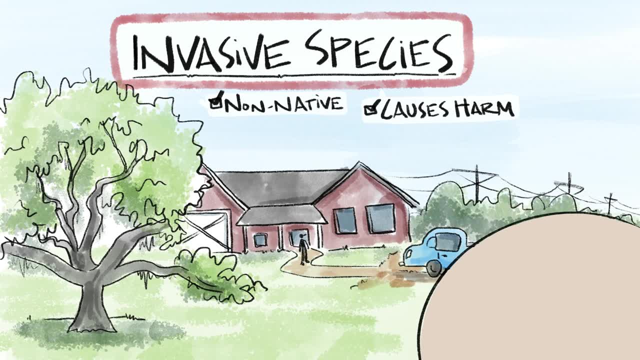 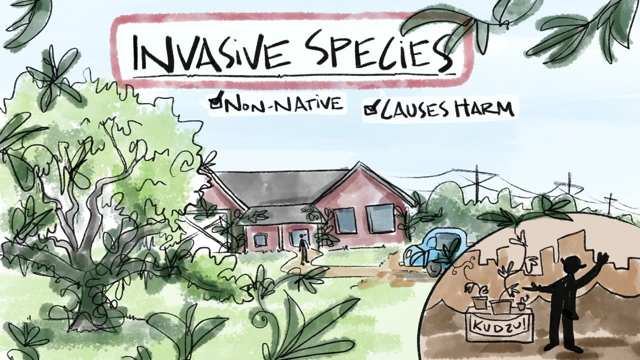 resources, infrastructure, economy, human safety and health, as well as plant and animal health. One example is kudzu. Kudzu was introduced to the United States in 1876 at an exposition in Philadelphia. It can grow up to a foot a day, allowing it. 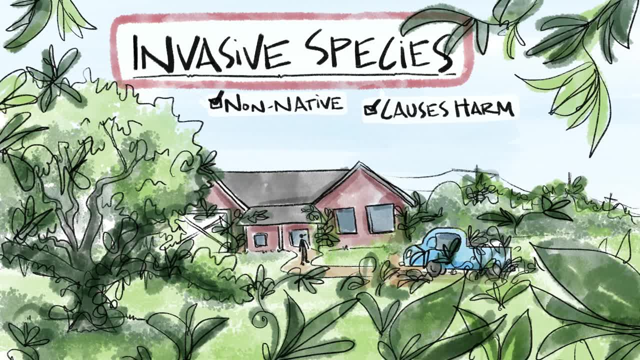 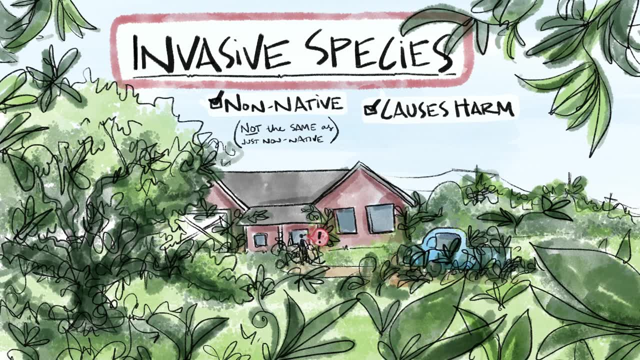 to easily out-compete and kill other plants. It even grows over power lines and poles, causing damage that results in the loss of power to communities. Now you may be thinking: where do pests fit into all of this? Great question, Let's.